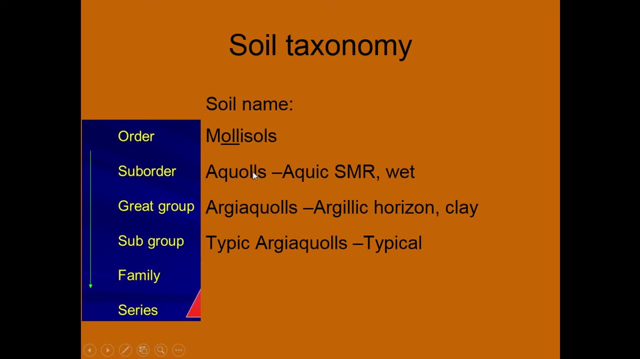 So then we have an aqual And then we have an argillic horizon in our aqual, So argillic is a clay deposit. So then we take the ARGI, So it's an argi-aqual, And then in the subgroup category there's sort of a flow chart of unique characteristics. 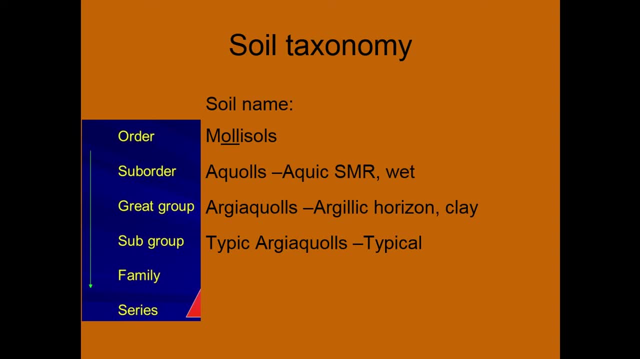 This one doesn't meet any of those. So it's just a typic argi-aqual, A typical argi-aqual, And so just in the classification, we know that it has clay deposit, A wet soil, moisture regime And it's a mollusol. 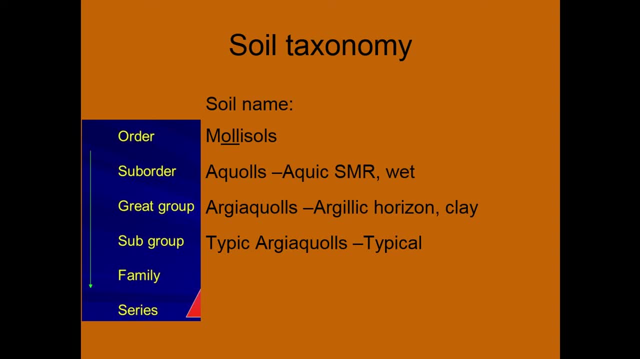 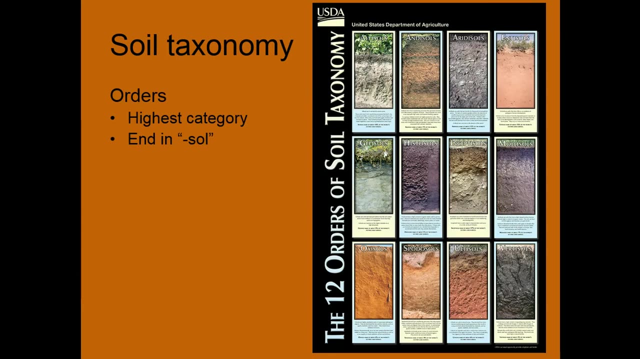 So it's one of our prairie soils with high organic matter near the surface. So that's how soil taxonomy works and sort of a unique thing compared to plant taxonomy. As mentioned, we have 12 soil orders. It's our highest category. 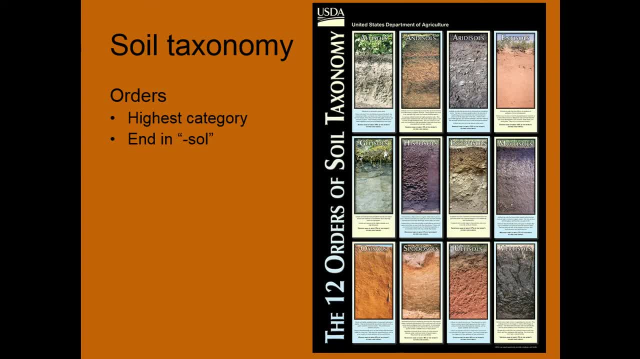 They all end in SOL or sol, So they are alfasol, andesol, eridosol, entesol, gelosol, histosol and septosol, Mollusol, Andesol, Oxosol. 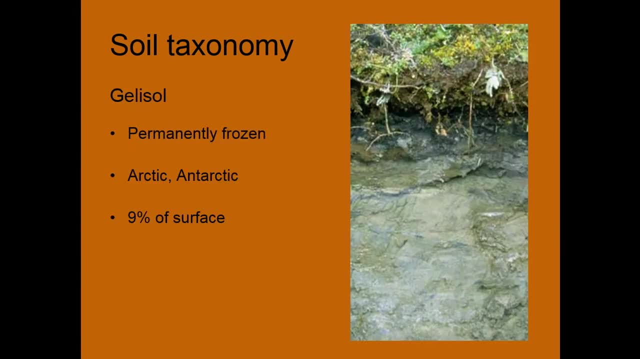 Spodosol, Altosol And vertosol, So we'll go through each one of these. So a gelosol is permanently frozen. These are found in the Arctic and Antarctic- About 9% of the surface of the planet. 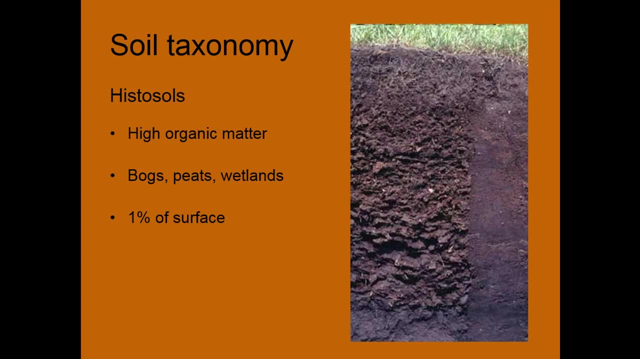 Our histosols are high in organic matter. These are like bogs, peats, wetlands, So really coarse organic matter that hasn't been broken down. They're often saturated- About 1% of the soil surface- but very important ecologically. 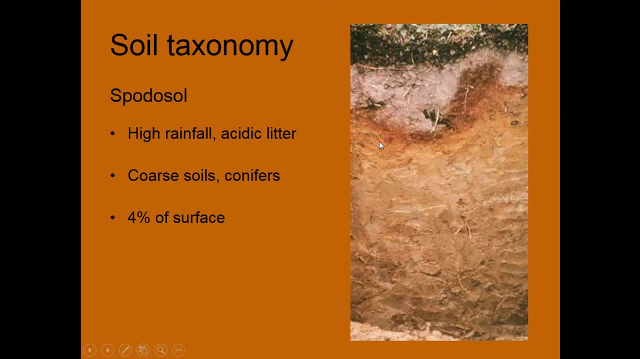 Spodosols are identified with the spodic horizon, So this is iron that's leached out and deposited, And this often has to do with pH. So we find these in coarse soils because we need lots of water movement And then high pH or low pH and then acidic litter. 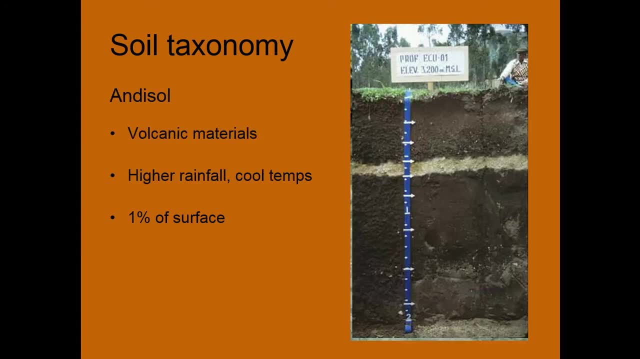 So often under conifer forests. About 4% of the earth's surface Andesols are derived from volcanic materials. A great place to see some andesols is if you ever get to go to Iceland, Make sure to check out the soil there. 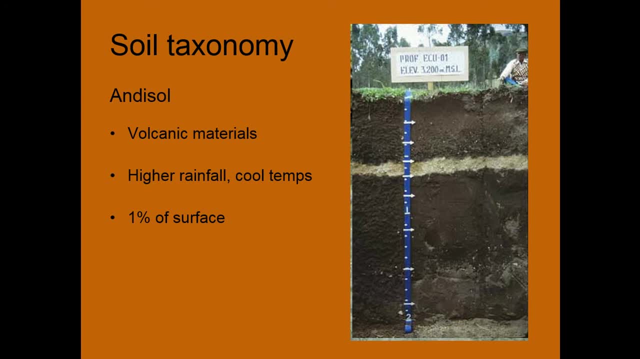 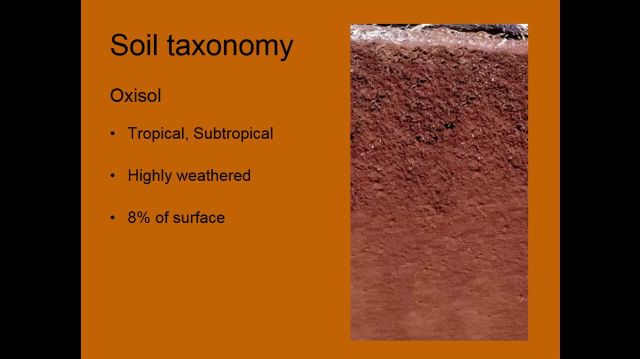 Higher rainfall content but cooler temperatures. About 1% of the earth's surface Axosols are found in tropical and subtropical areas. These are really red, Sort of like a typical rainforest Soil that you see in pictures. They're red because they're highly weathered. 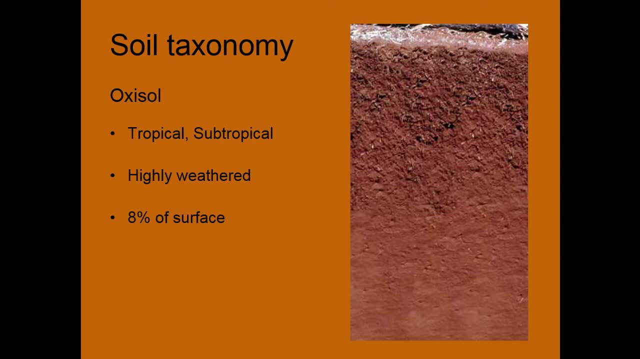 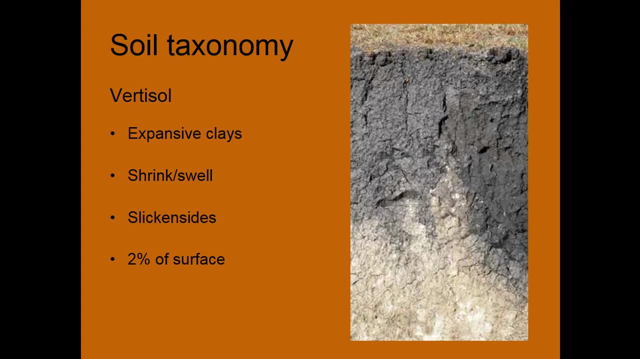 So that's clay content And iron left over in the soil And about 8% of the soil's surface Vertisols. These are expansive clays, Which means that the clay present. they have a high chance of shrinking and swelling based on soil moisture. 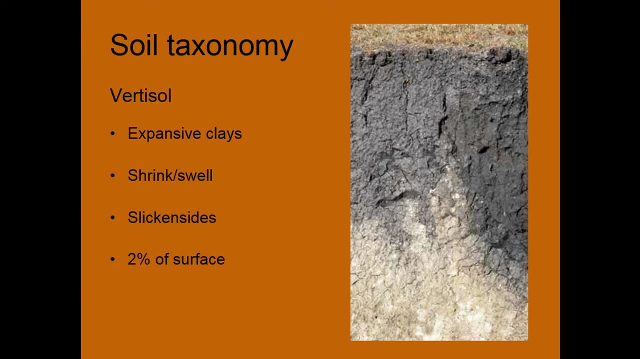 This creates slickensides, Which is a unique soil structure As a result of that clay kind of shrinking and swelling on each other and then sliding, And it's about 2% of the soil's surface. These can be found in Texas, in the US. 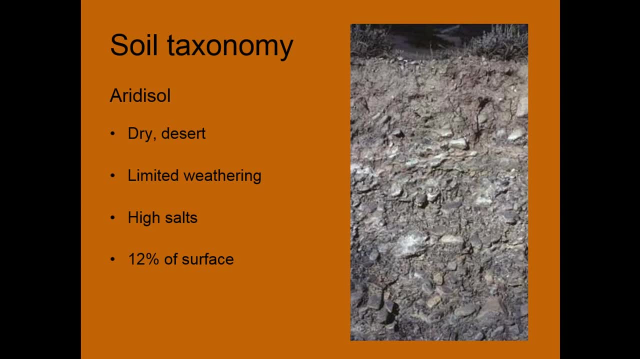 It's probably our best region for them. Up next we have aridisols, So arid. So these are our dry desert soils. They often have limited weathering because of the low moisture And then high salt content Because we have water moving up through the soil profile. 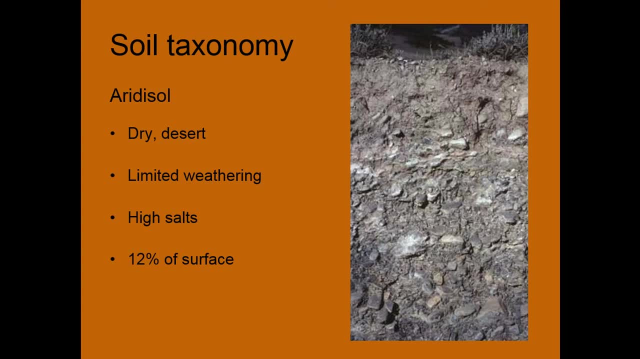 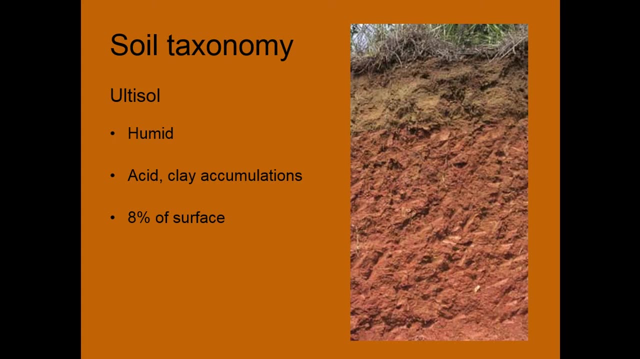 And then evaporating at the surface, leaving behind that salt, And then they cover about 12% of the planet's surface. Altisols are found in humid areas. They're often acidic And have these clay accumulations which you can see in the red color. 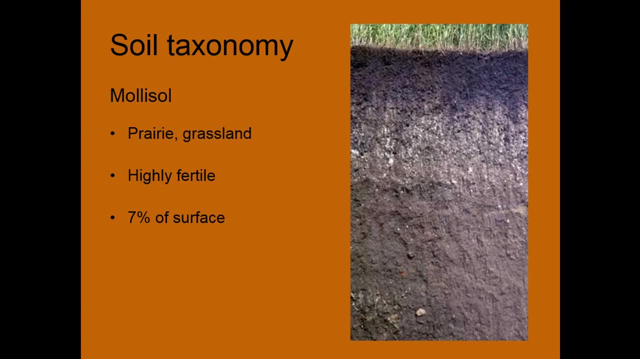 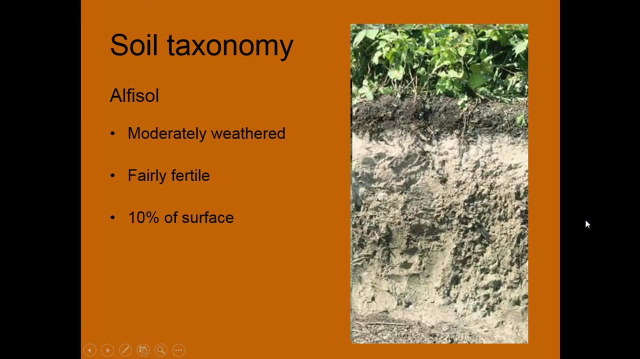 About 8% of the soil's surface: Mollisols. These are our prairie or grassland soils. They're highly fertile Due to this very rich and deep organic matter horizon here Which we use to identify them: Alphasols. 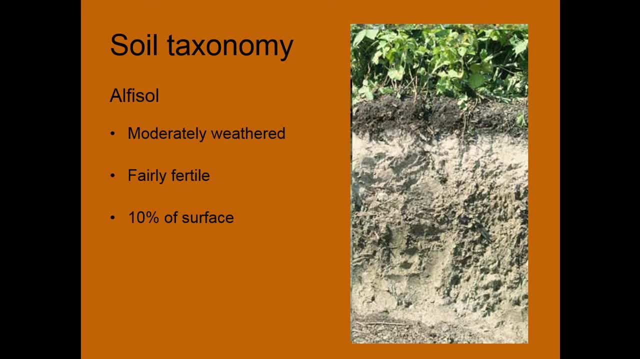 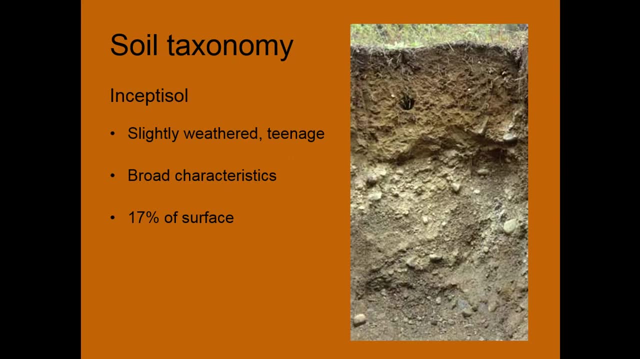 Moderately weathered, Fairly fertile, A lot of our farmland And covers about 10% of the soil's surface. Then we have enceptosols, Which are slightly weathered, So that means they don't quite have as clear horizon definition. 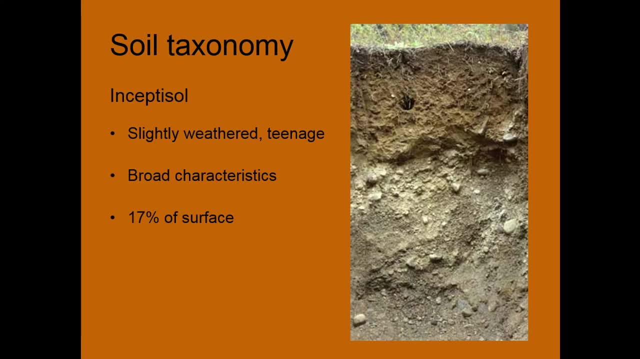 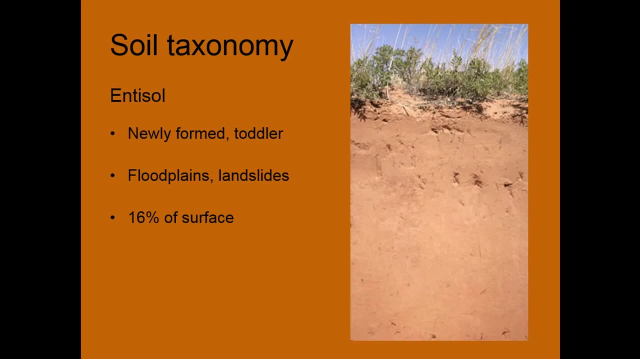 Usually fewer horizons, Broad characteristics, Sort of our teenage soils, Geologically speaking, And then our entesols. So these are like our baby soils, Our toddler soils, Newly formed. Very few horizons, if any, Often as a result of flood plains or landslides. 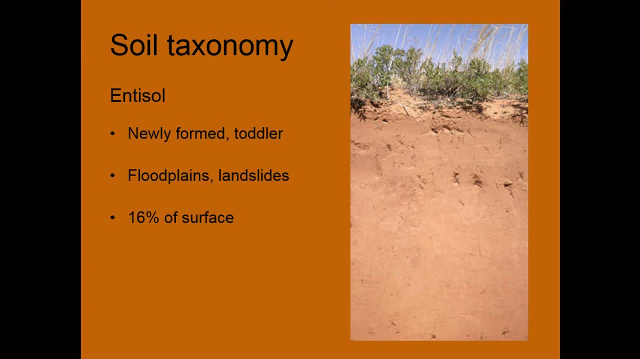 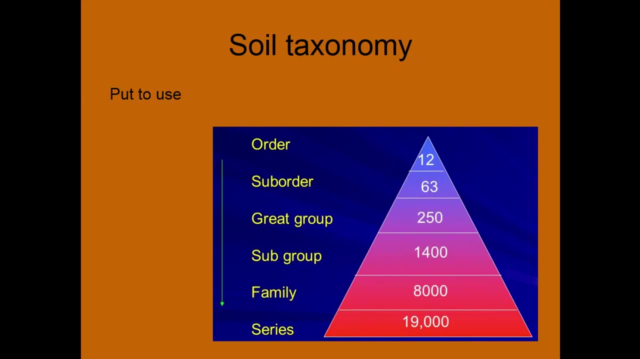 So recently deposited And the soil forming factors are clorped, Hasn't had very much time to act on them. So now, if we go back to our hierarchy of soil taxonomies, Then we can put it to use in an example here. 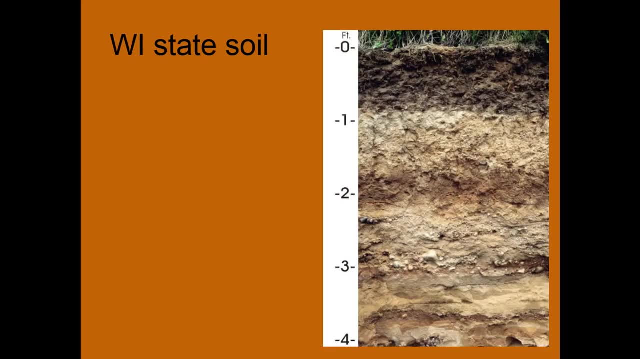 We'll do the Wisconsin state soil, So I'll give you a second to remember what the Wisconsin state soil is. First of all, here's a picture of a profile for it And, as you all remember, it's the anago silt loam. 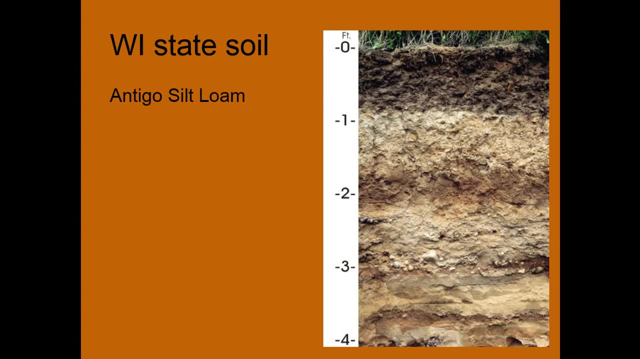 There's a song about it. If you need help remembering it, You can search online for that. So it's an alfasol. So we take the alf off of that. It has a eudic soil moisture regime, So it's a eudulf. 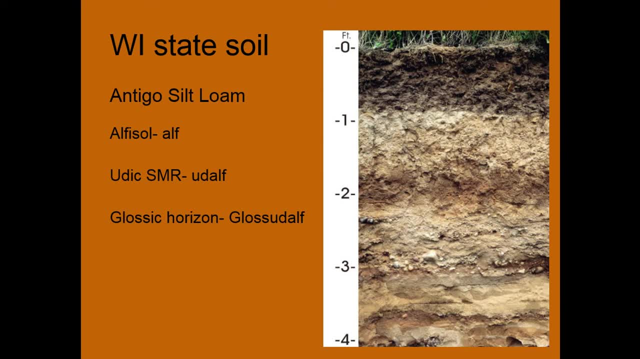 And then it has a glossic horizon here, So it's a gloss eudulf, And the glossic horizon is less than 50 centimeters thick, Which makes it a haplic, And it has a frigid soil temperature regime Which is just based on how long the soil is cold. 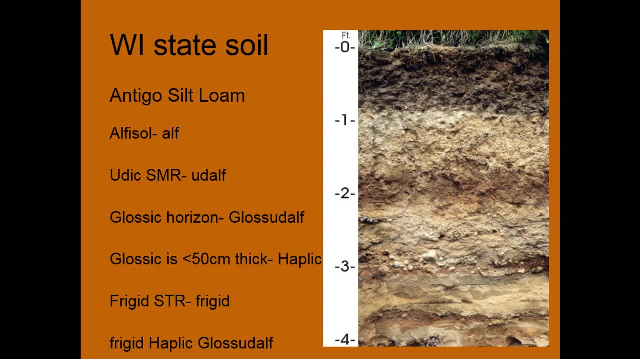 At a certain depth. So all in all, our Wisconsin state soil, The anago silt loam, is a frigid haplic gloss, eudulf, And then we can sort of pick out some horizons here. And so this is what we do. first, 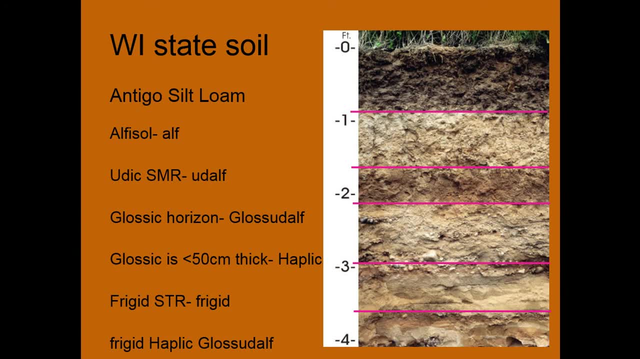 We would identify the horizons And then key it out to a frigid haplic gloss, eudulf. So we're working a little bit backwards, But these are our rough horizon boundaries. Then we have our master horizons. We don't have an O horizon here. 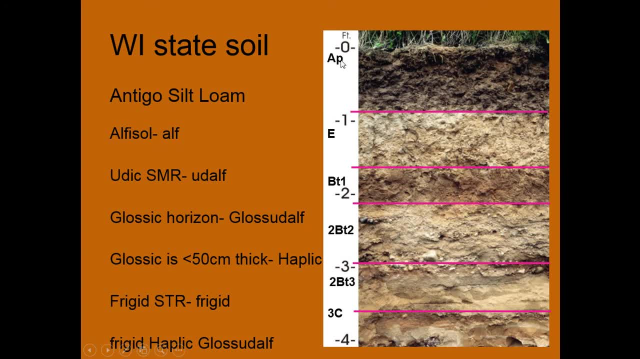 We just have an A And then the small p denotes a plow layer, So AP. Then our light layer, here Is our zone of eluviation, Or E horizon, And then the clay that is eluviated out of here. 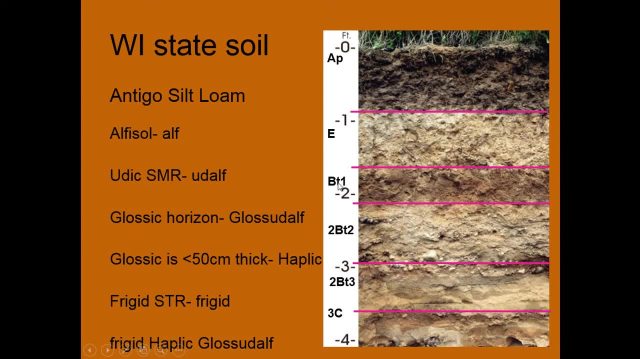 Gets deposited into our BT horizon, So the T here denoting a high clay content, And then we switch to a 2 BT horizon, 2, BT, 2.. The 2 at the beginning denotes a different parent material. So a lot of times in Wisconsin we see this: